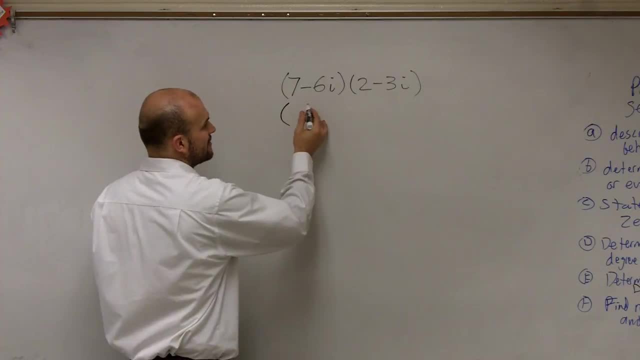 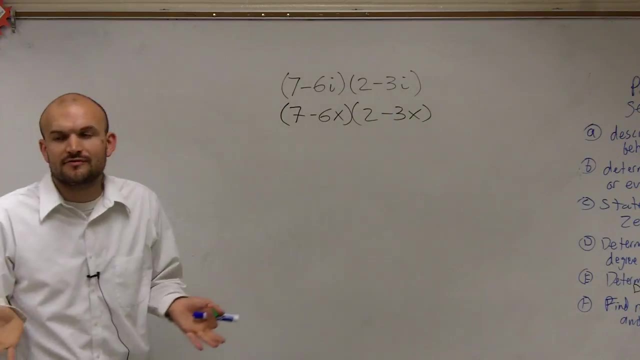 about this is when you're multiplying. think of this as 7 minus 6x times 2 minus 3x. alright, Just think about it. forget about the i for a second and forget about all the properties of i. just treat it like a variable and our most common variable that we could use. 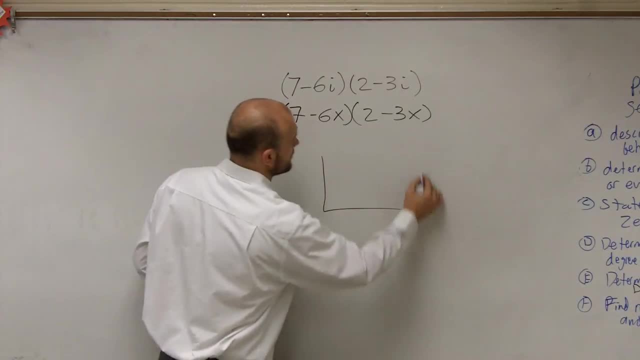 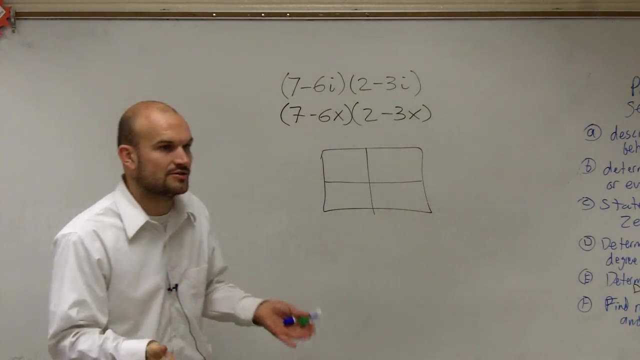 was x. So when we multiply- alright, if I was going to multiply these two binomials- the best way that I like to do it to keep everything organized is to create a box And because, remember, when multiplying two terms, you're really creating an area. So what I 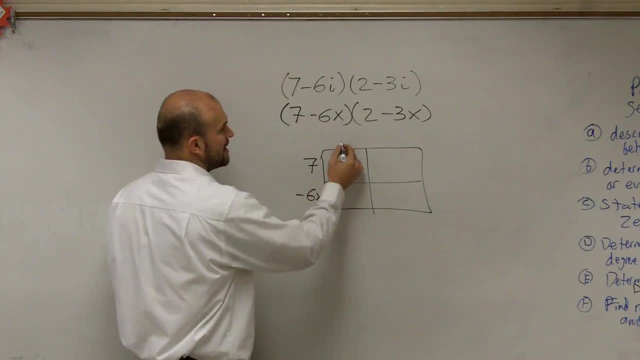 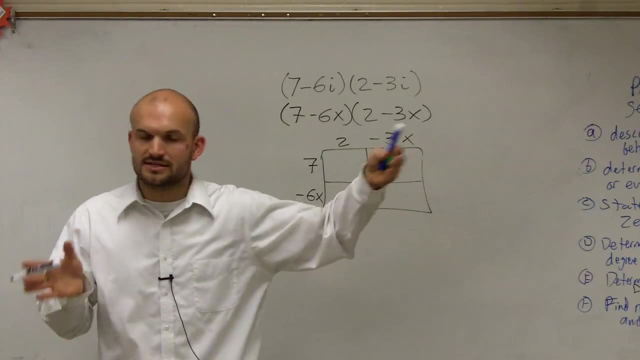 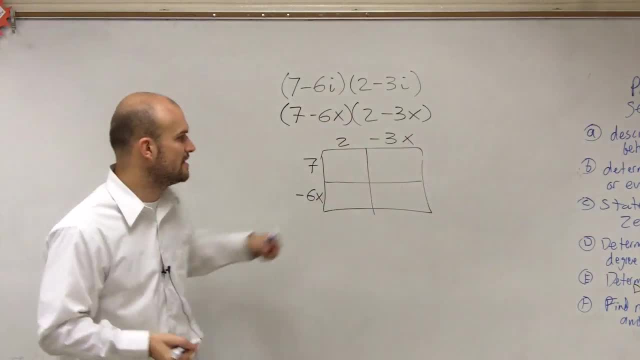 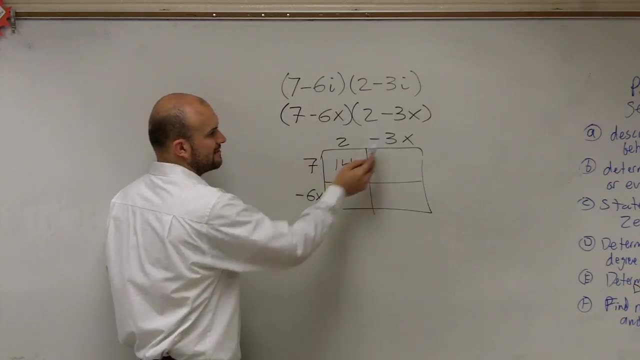 it's a binomial. I break up my box into two different sections. Then all you do is multiply your length times your width for each box. So 7 times 2 is 14,. 7 times negative 3x is going to be a negative 21x. 2 times negative. 6x is negative 12x and negative 6x times. 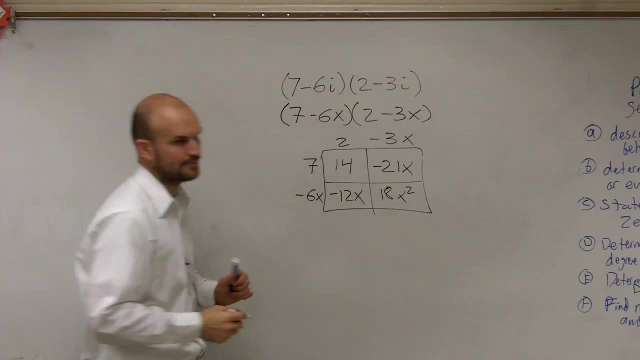 negative 3x is a positive 8x squared. And the cool thing about yes, Positive 18x squared. Okay, I'm just going to go back with the i in just a second. X times x is x squared, Alright. 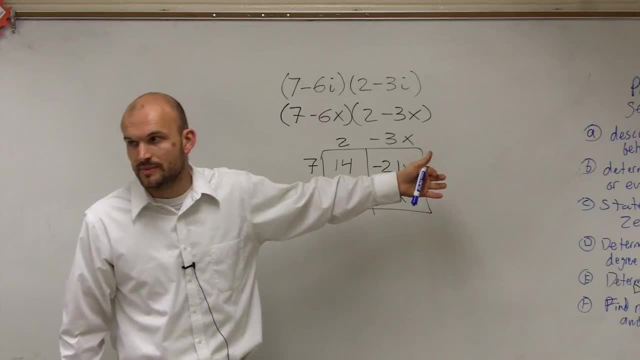 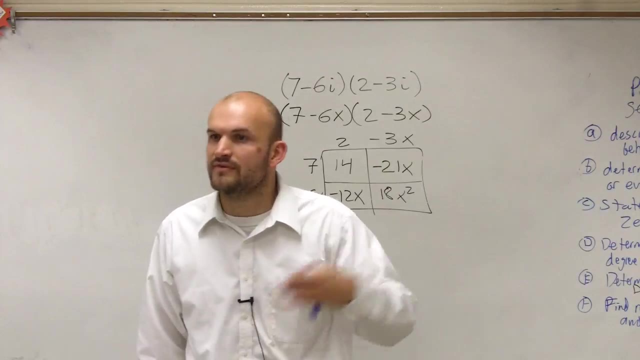 A number multiplied by itself is going to be squared, So it would be: x times x equals x squared, Just like: 3 times 3 is 3 squared, right? What's 3 squared? It's 3 times 3.. So 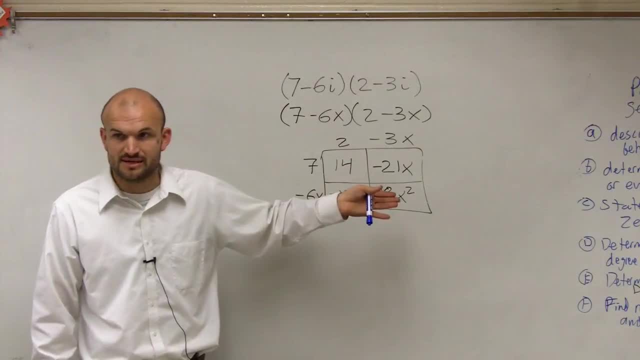 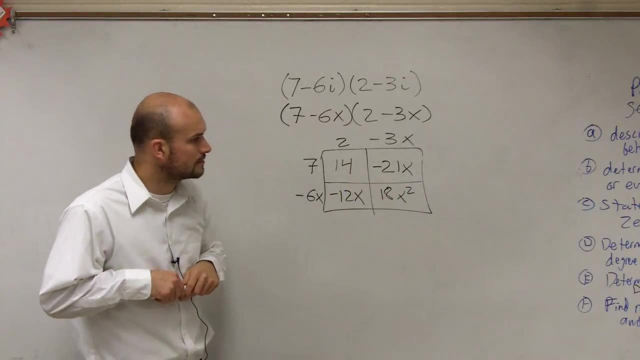 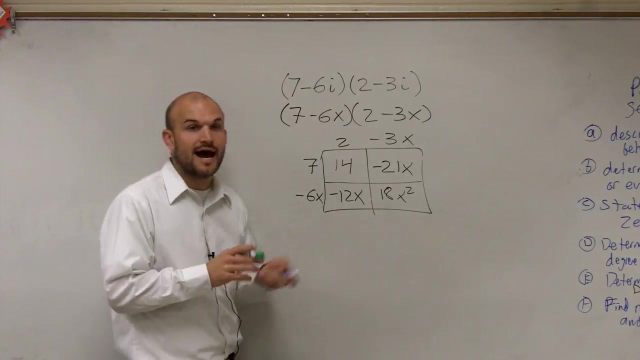 if I have 3 times 3, that's going to be 3 squared. So x times x is going to be x squared. Does that make sense? I'll go and do another example here in a second. Now here's our problem. Our i, we're not. 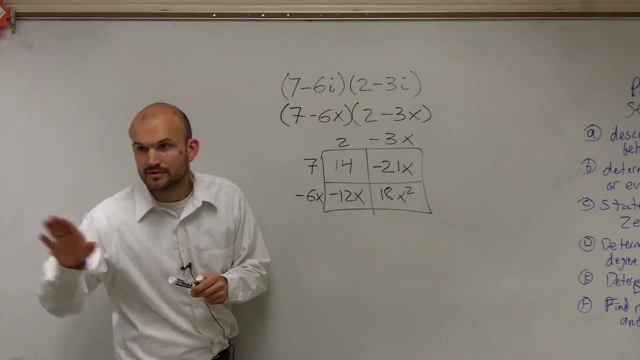 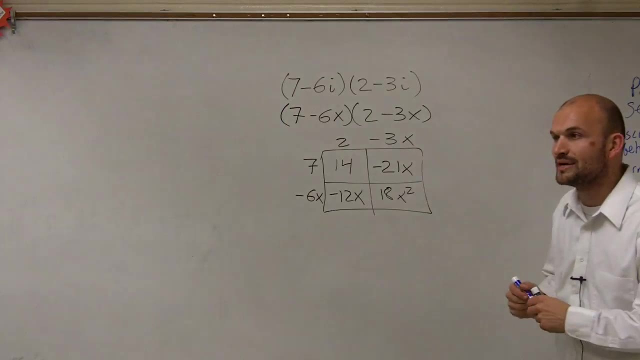 including our i in this? have we Terrell? Okay, Because I'm going to ask you to have to sit back there if you can't just pay attention to this. okay, So we haven't used the i yet, alright, So to incorporate the i just kind of replace the x's with the i's.